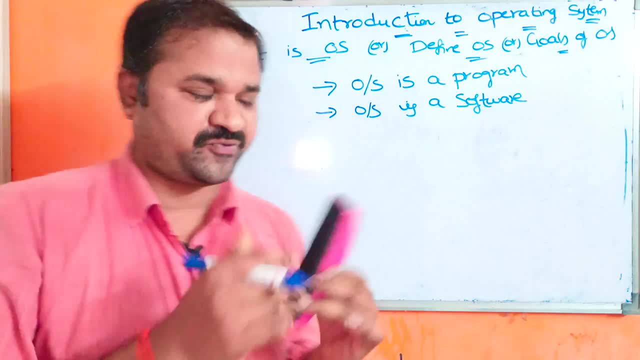 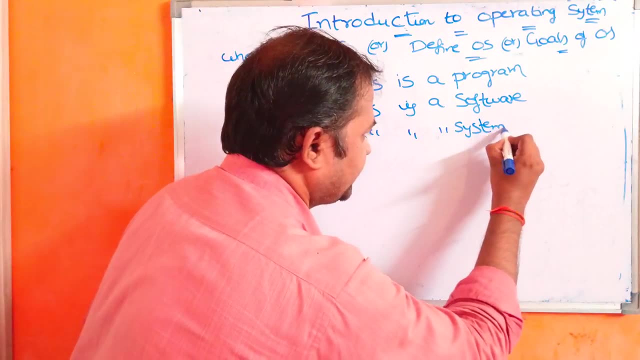 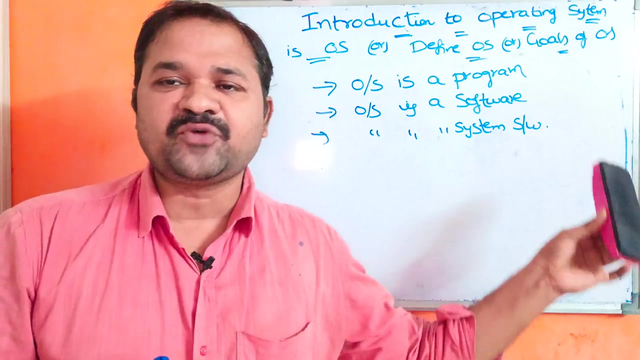 Whereas operating system comes under system software. So operating system means it is a system software. So what is a system software? We can use the system, We can use the computer In effective manner with the help of the system software. Operating system is a system software. 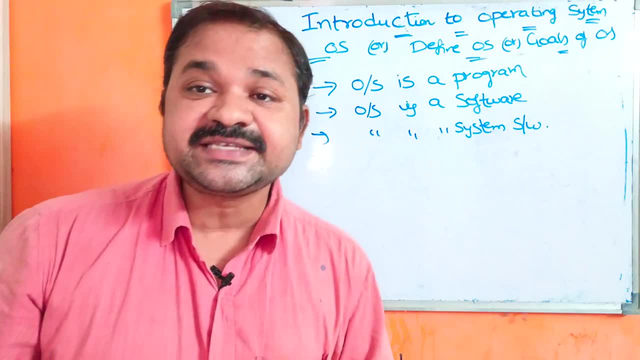 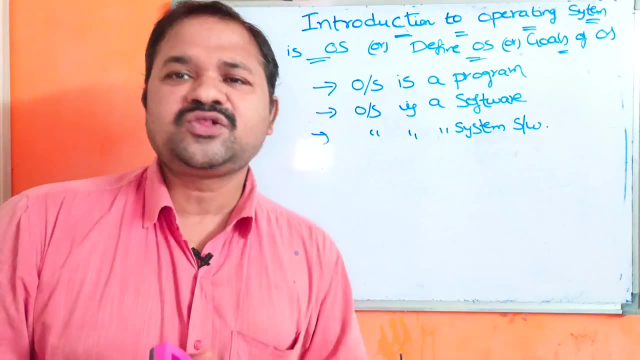 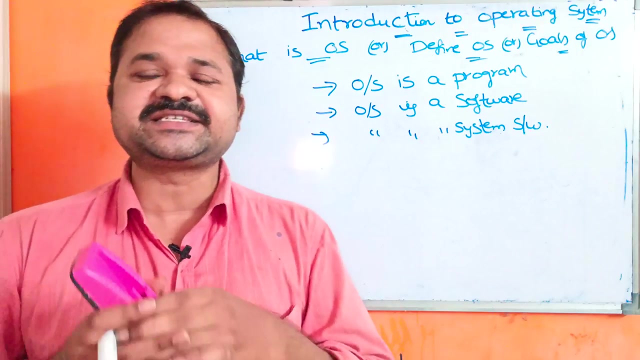 Compiler is a system software. Assembler is a system software. Text editors are some system softwares, such as notepad, wordpad. All those are system softwares. We can utilize the computer in effective manner. So operating system means a system software. Now let us see the definition. 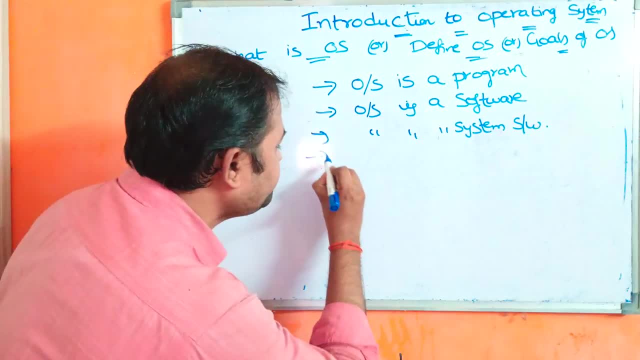 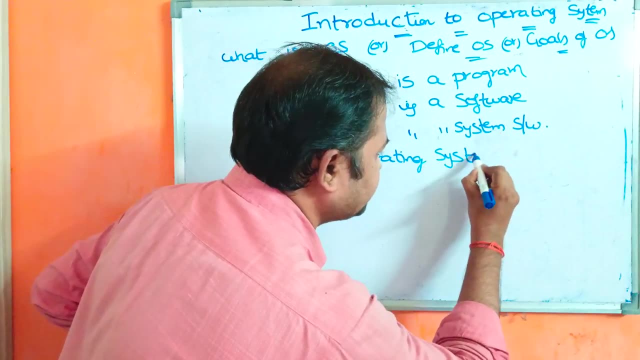 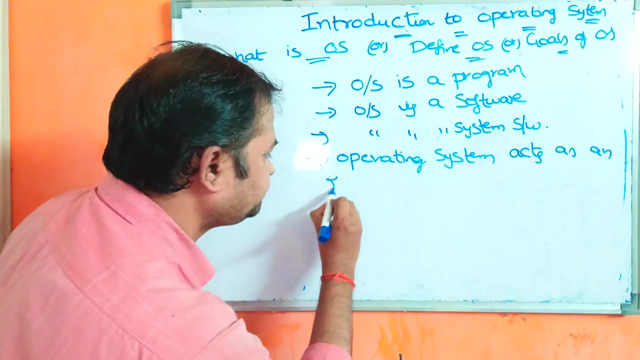 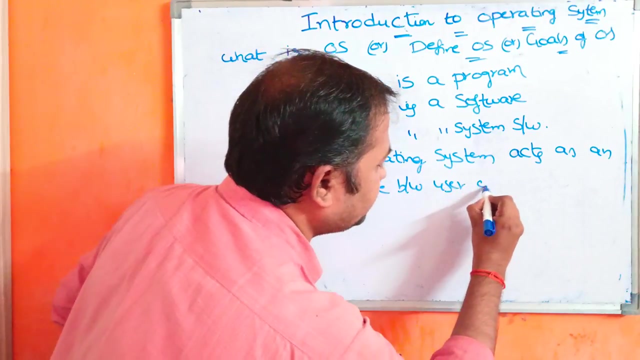 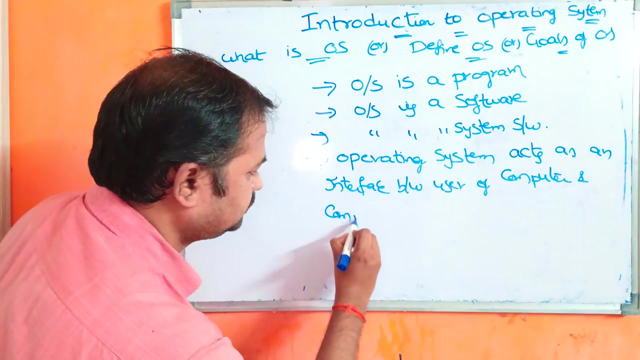 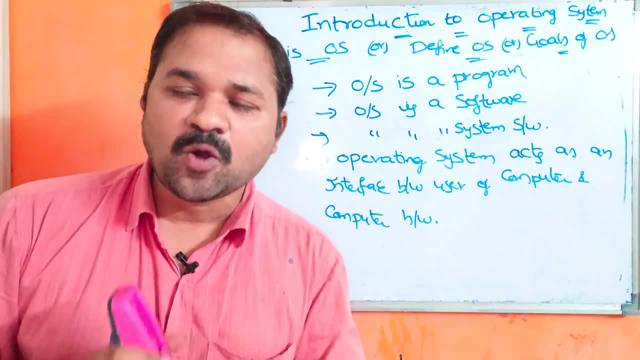 So operating system acts as an interface between user of computer and computer hardware. So operating system acts as an interface between user of computer and computer hardware. So operating system acts as an interface between user of computer and computer hardware without installing the operating. without installing operating system we can do an. 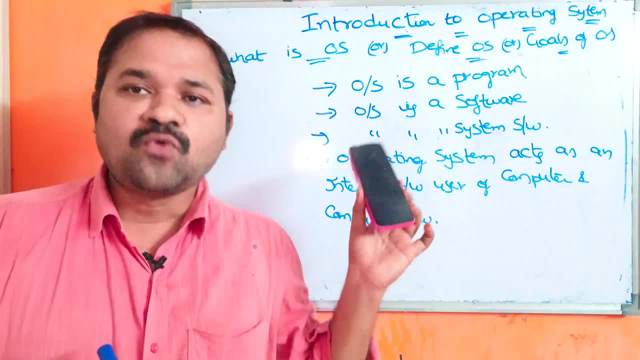 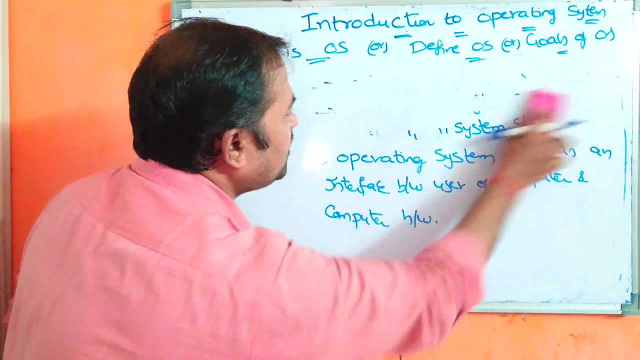 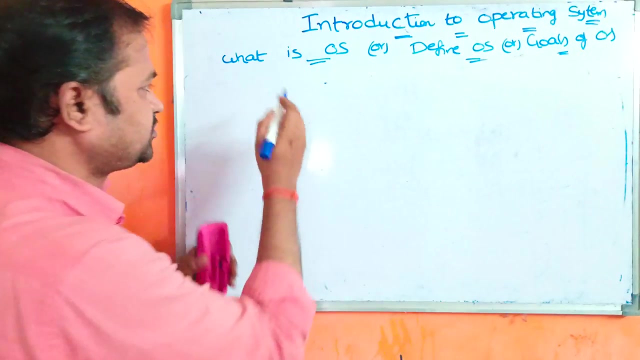 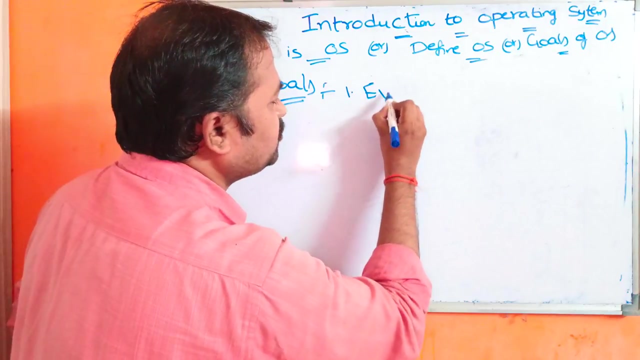 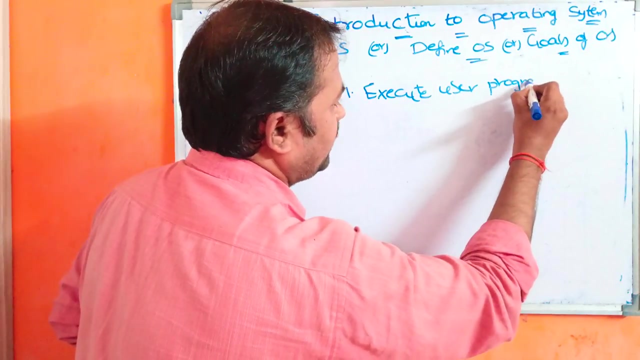 activity or several activities in the computer only by installing the operating system. now let us see the goals of operating system. so what are the various goals of an operating system? mainly we have three goals, are there? let us see those three goals. so goals of operating system. the first goal is: execute user programs. execute user programs. execute user programs. the second: 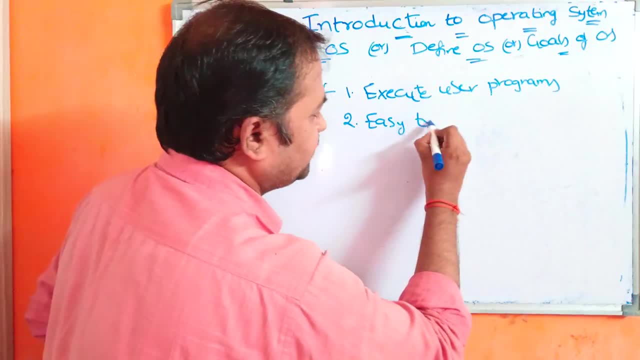 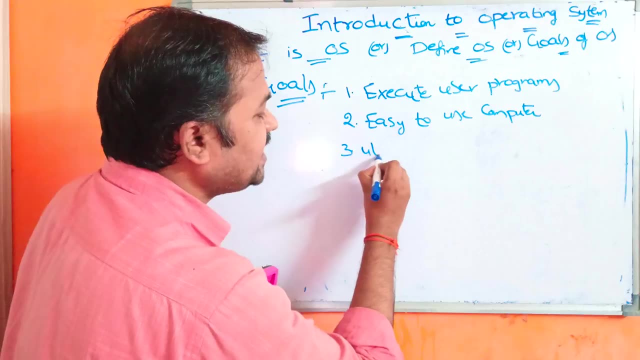 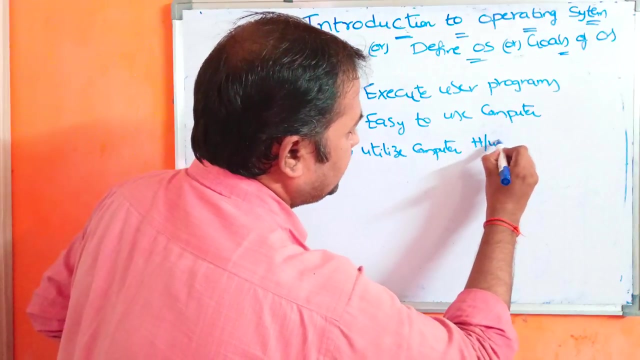 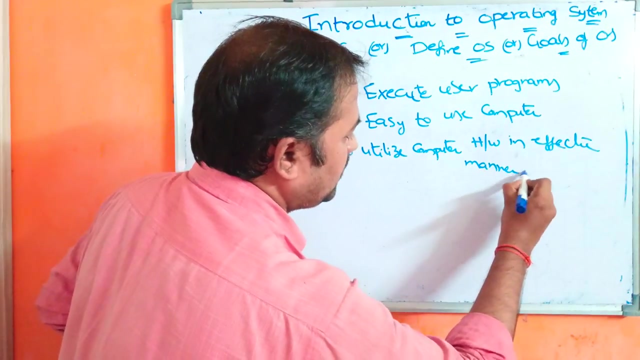 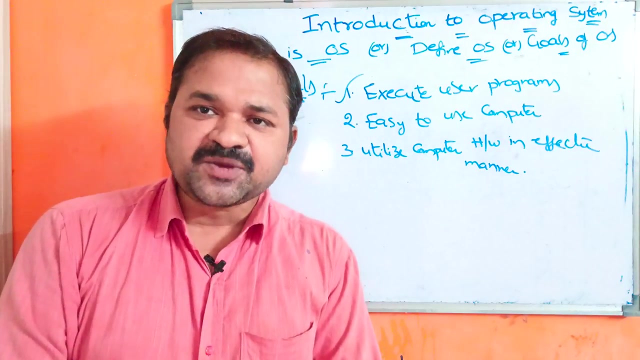 goal is easy to use computer, easy to use computer. the third goal is utilize, utilize computer hardware, computer hardware in the effective manner. in the effective manner. let us see these three goals now. the first goal of the operating system is execute user programs. operating system provides an environment to 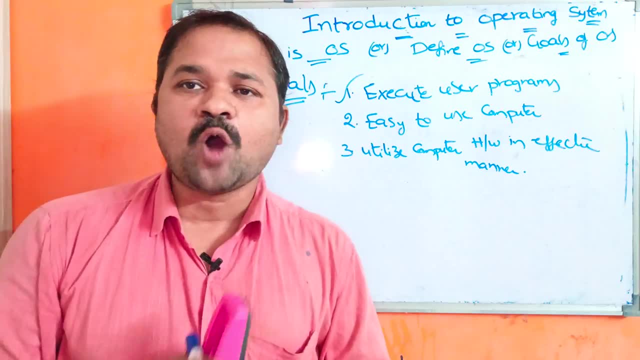 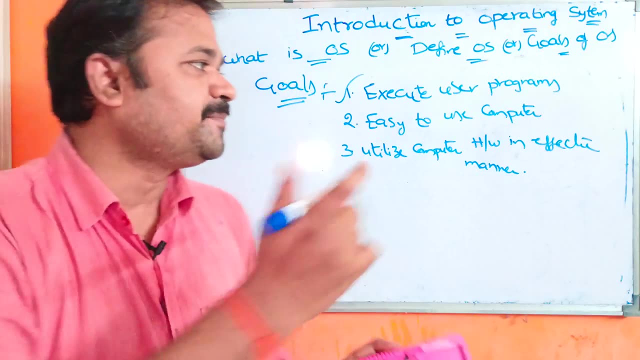 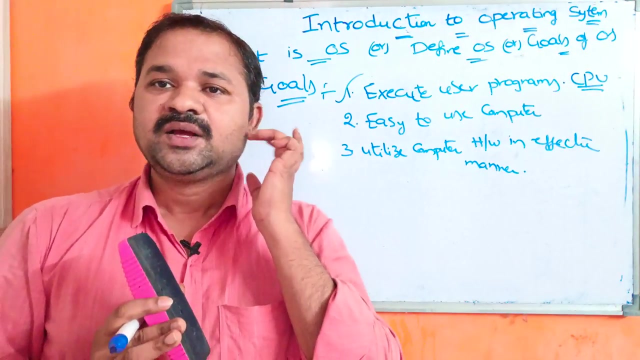 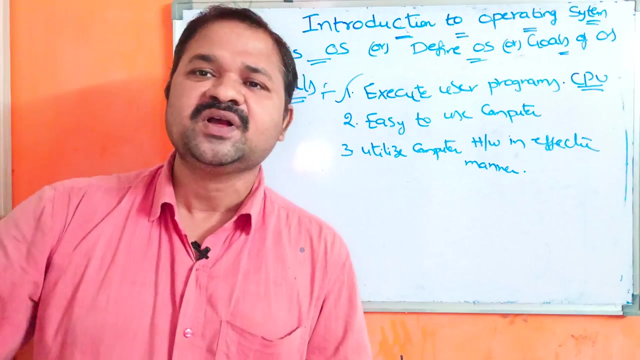 execute the user programs. actually, operating system cannot execute the program. a program or any task is executed by CPU central processing unit. that is nothing but a processor. okay, generally, if you take any programming language, it may be C or C++ or Java or Python or C, sharp JavaScript, any programming language. 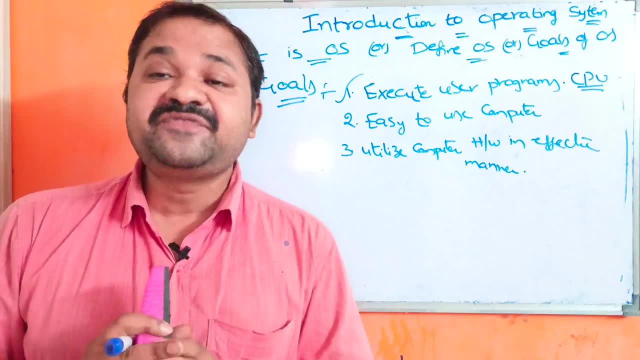 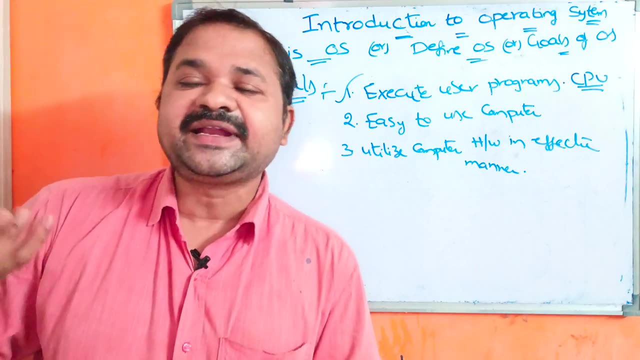 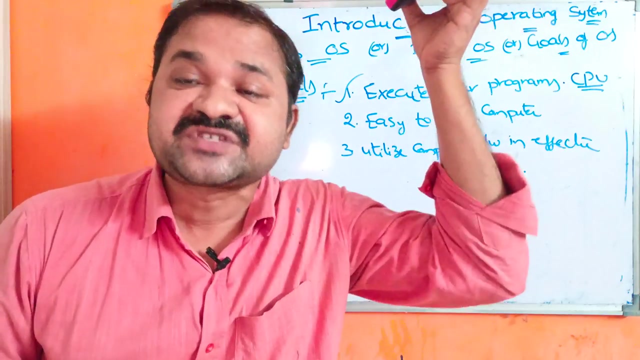 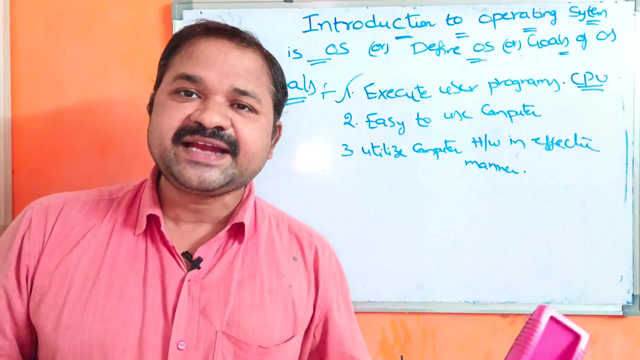 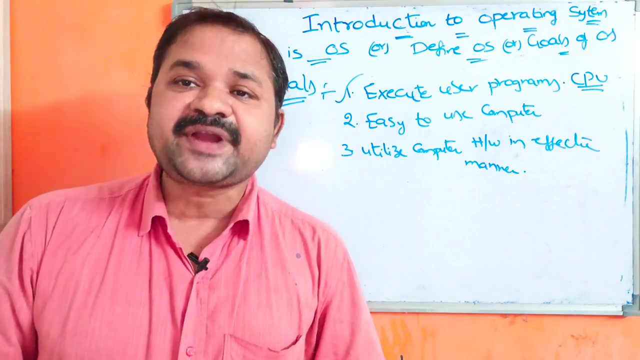 if we, after typing the program, if you save the program, the corresponding program will be saved in hard disk. that is nothing but secondary memory. so whenever we save the program, the operating system saves the program in hard disk. during compilation also, the program will decides in hard disk only, but at the time of execution operating system transfers the program from hard. 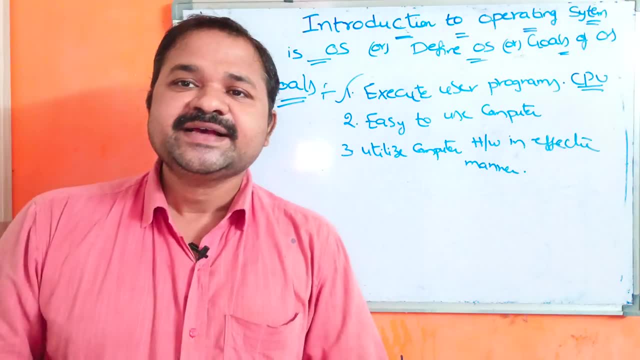 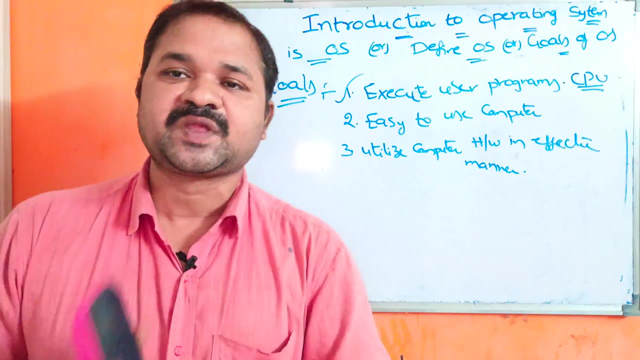 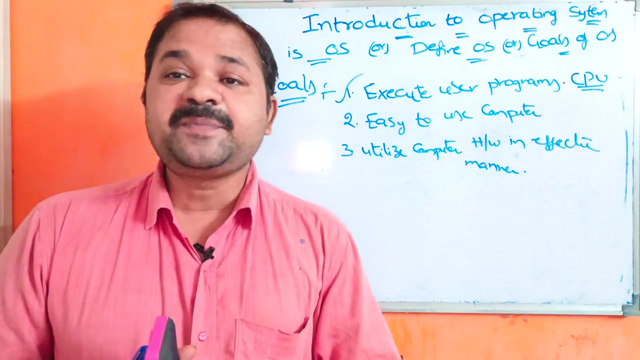 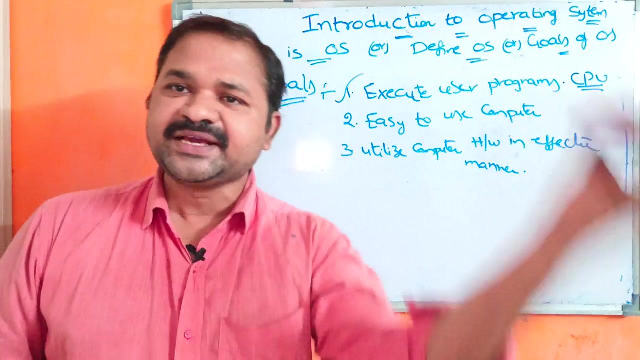 disk to main memory. why? because CPU can execute a program when the program resides in main memory only. CPU cannot access secondary memory. CPU cannot access hard disk. CPU can access only main memory only. so saving the program in hard disk, transferring the program from hard disk to main memory after. 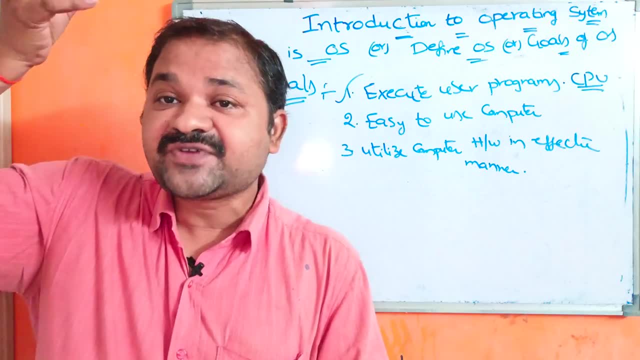 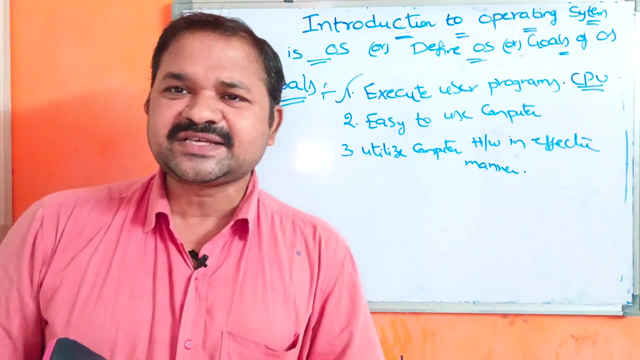 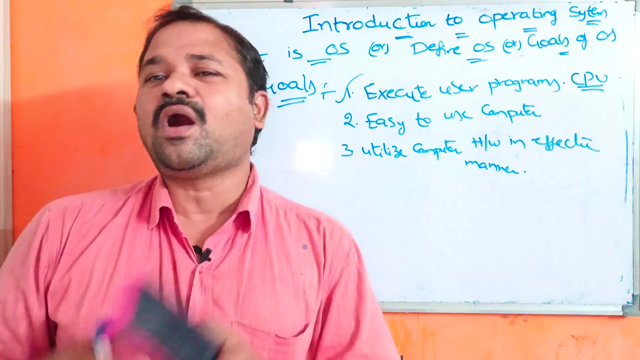 execution is over. once again, that program will be transferred from main memory to the hard disk in order to save some other program in the main memory. why? because the size of the main memory is very, very small. main memory can store only limited number of programs, only okay, so, uh, so all those things are done by operating system. 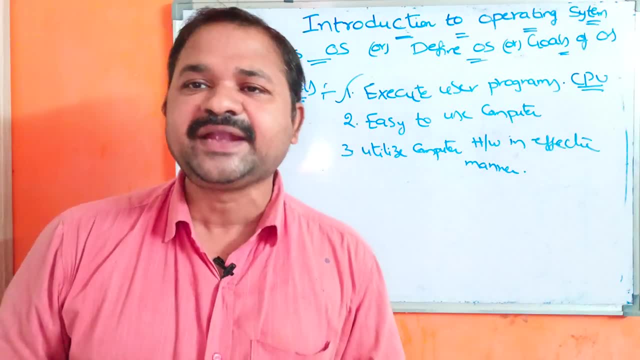 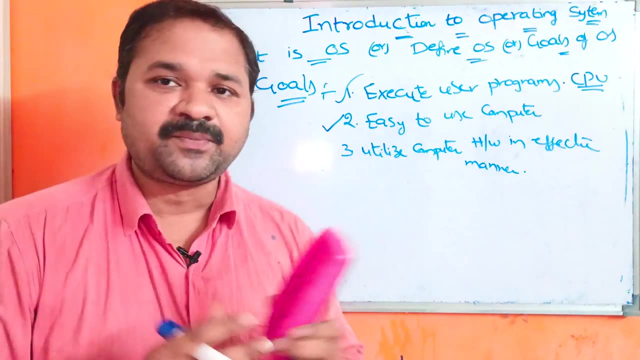 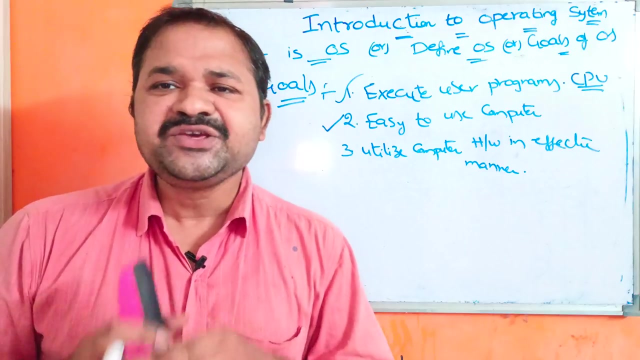 only so operating system provides an environment in order to execute the programs. now let us see the second program. second goal: easy to use the computer. we can use the computer in effective manner only with operating system as a user. let us assume that we have given some printout now. 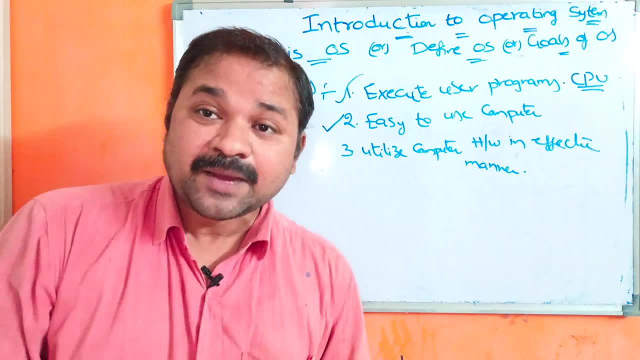 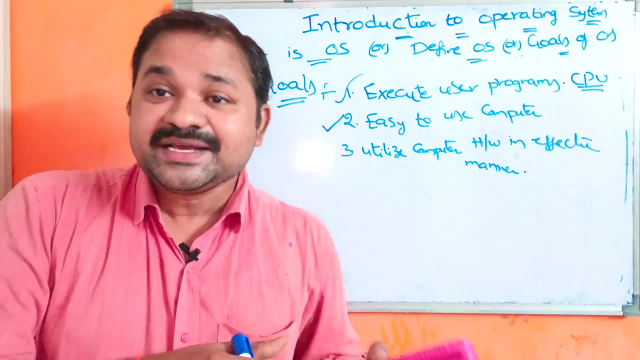 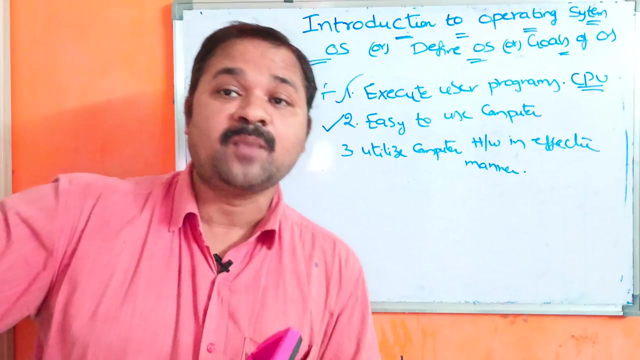 it is the duty of the operating system to allocate printer. as a user, we have- uh, we have done some scanning. okay, it is then now also it is the responsibility of the operating system to allocate scanner to our program, to allocate scanner to our file. so everything will be taken. 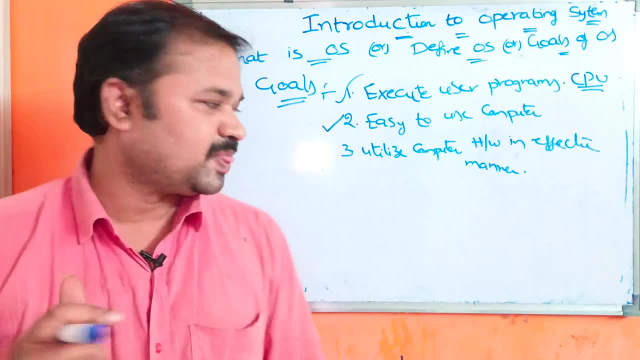 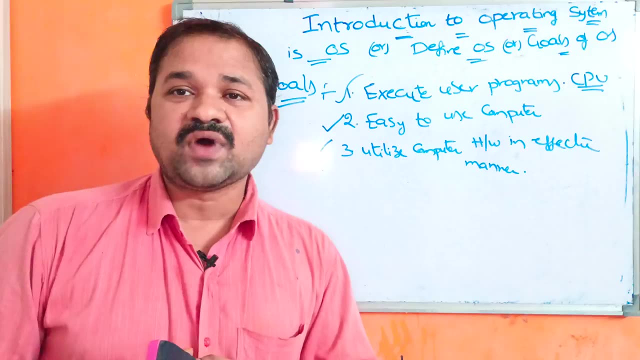 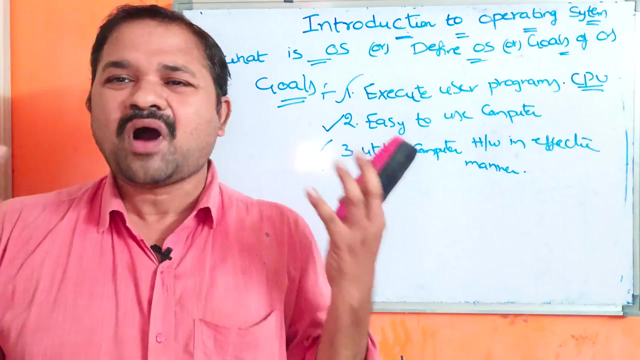 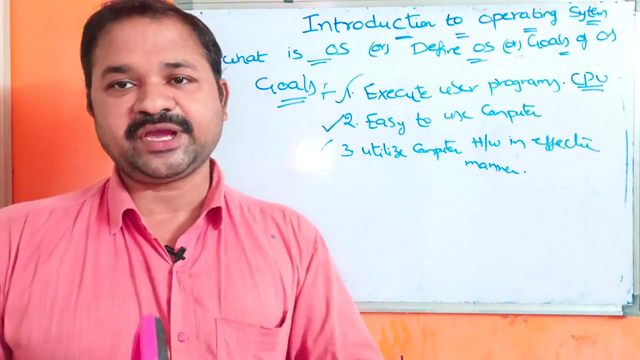 care by the operating system only. we should not worry about that. and let us see the third advantage: utilize computer hardware in effective manner. so we have various hardware components such as ibot devices, so keyboard, mouse, printer, scanner. so all those hardware components will be utilized more effectively only with operating system only. okay, so these are the major goals of operating system. 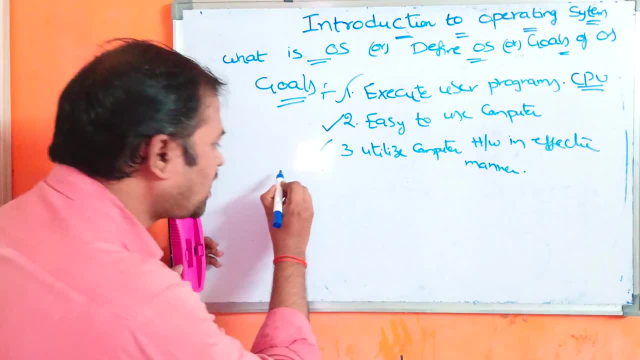 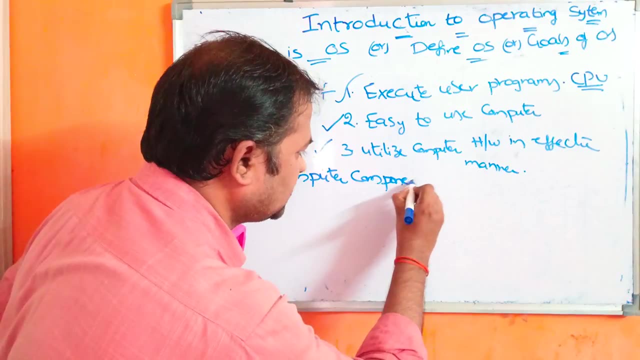 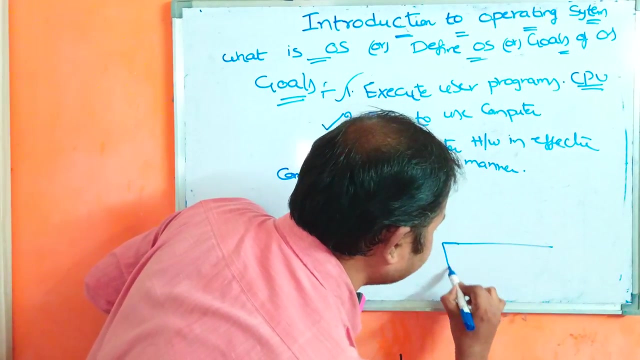 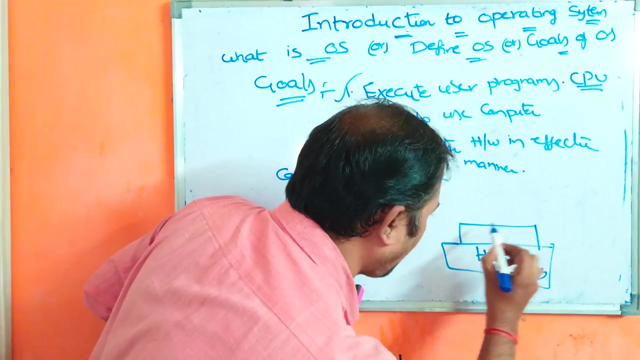 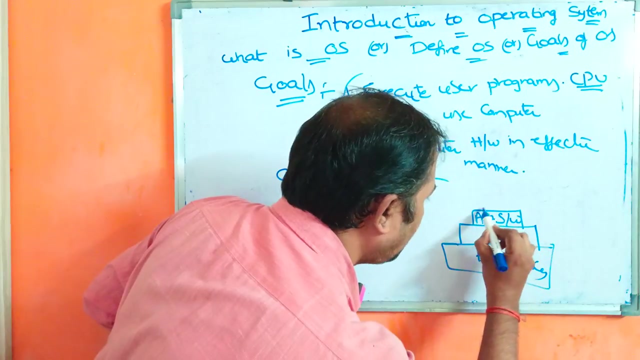 now let us see the components of the computer. computer components here. computer mainly contains four components. the first component is, so at the top we have hardware devices. next, on top of the hardware devices, we have operating system. on top of the operating system, we have application software. on top of the application software we have users. so hardware. 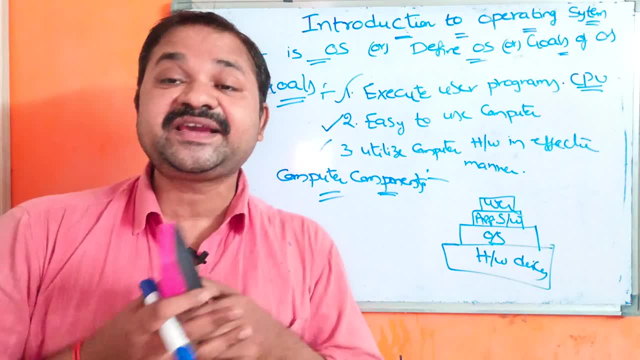 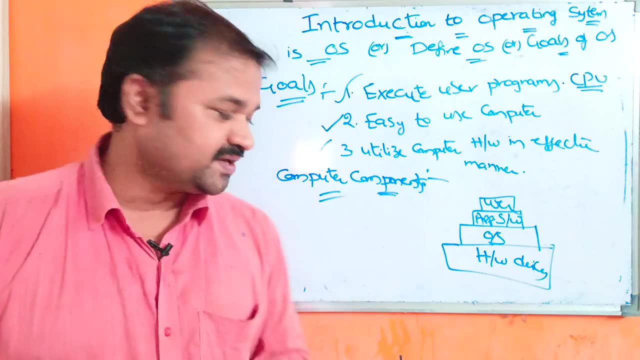 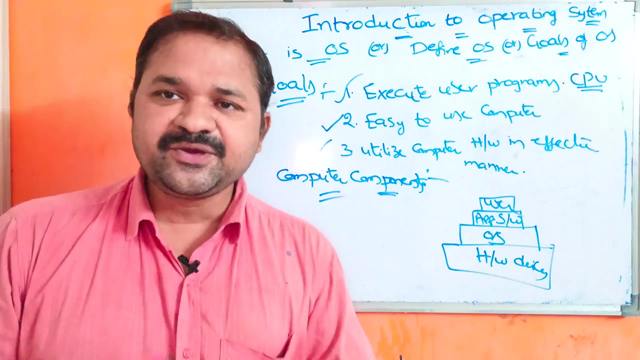 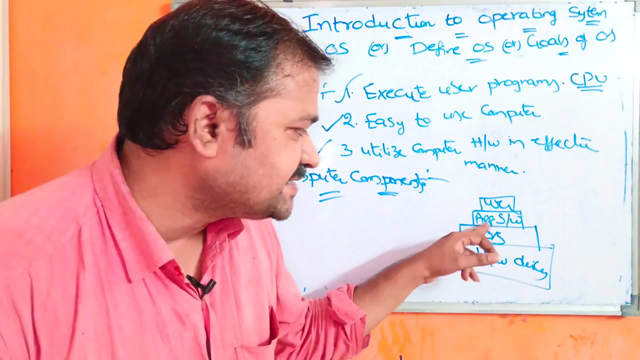 devices already we have seen. so hardware means the physical components of the computer. so we have application software, application software. application software means the programs which are developed by the user. so user develops the application software letter. so this effect, GitHub software application, software application in this can be done on a computer if you use a mobile computer. 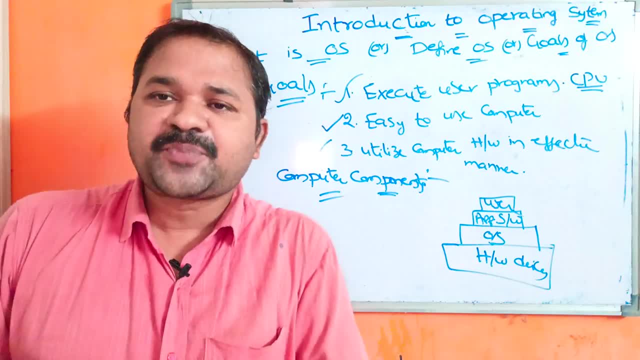 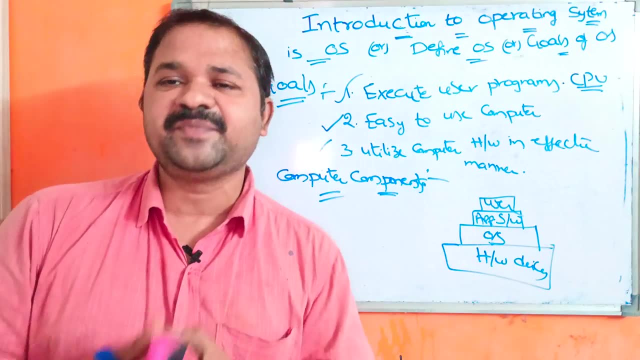 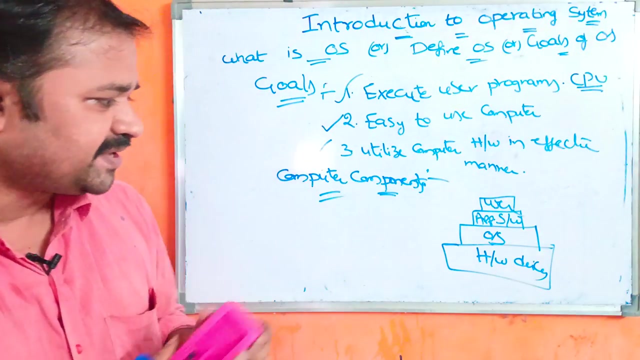 so we haveoud Firefox, Microsoft, but text. so this application software, Content, application software software. application software. application software grants on top of the operating systems app software. so on top of operating system we have application software. application software means the programs which are developed by the user. so user develops the application software for the requirement. so according to their requirement they will develop the application programs. so these are the major components of the computer. so in the subject to be 01.04, Ma não é um alh, returns to do0, fundamental software. �arf danился sem preparação. 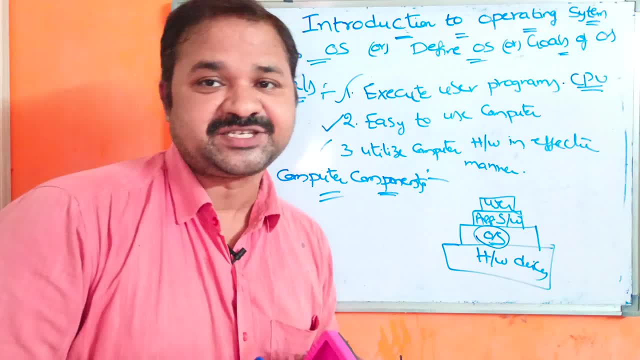 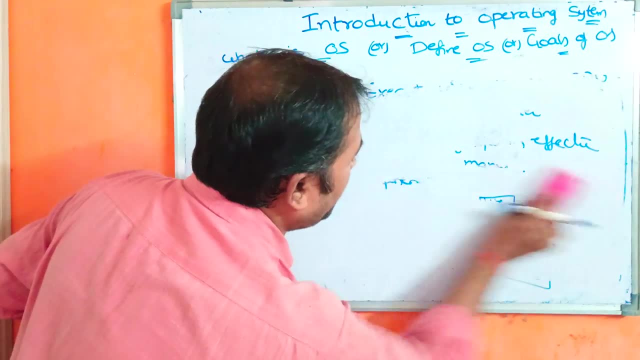 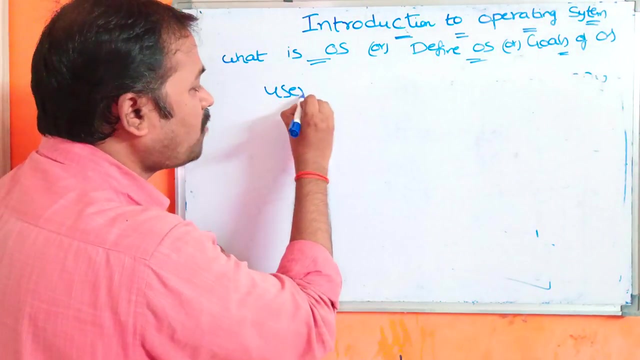 the second component, that is nothing but operating system. now let us see what is operating system from user point of view and from system point of view. so, from user view and from system view, what is an operating system? what does an operating system will mainly do from user view, from user? 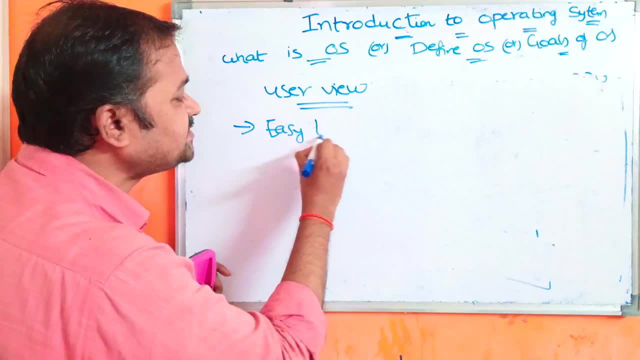 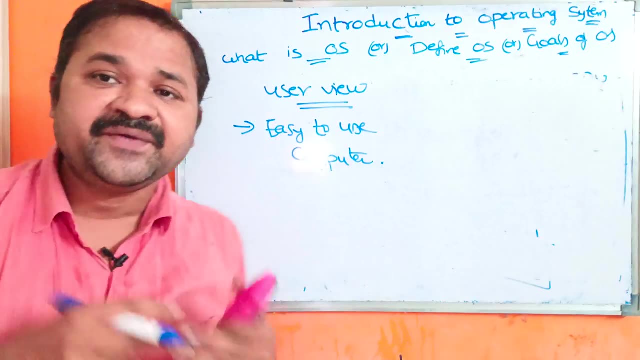 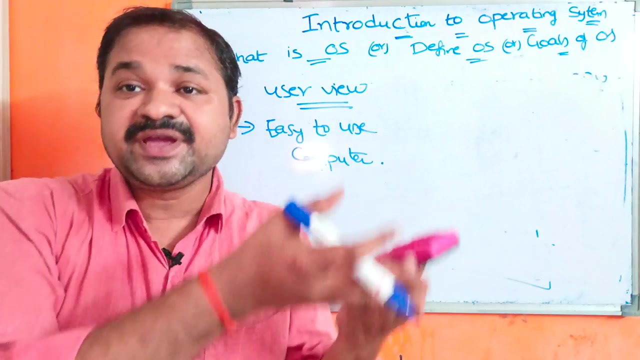 view, the major advantage of the operating system is easy to use computer. so by using operating system we can use the computer very, very easily. if you type the program and if you save the program then so compilation during compilation. the program resets in hard disk only during execution. 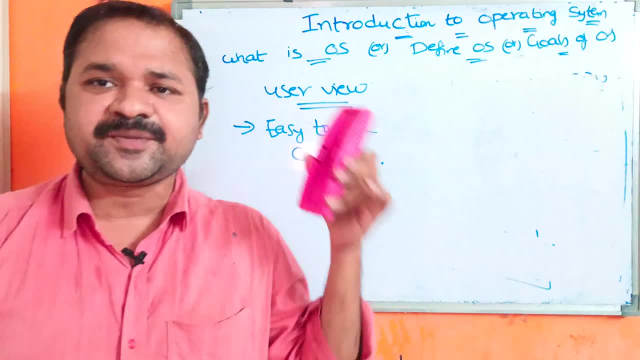 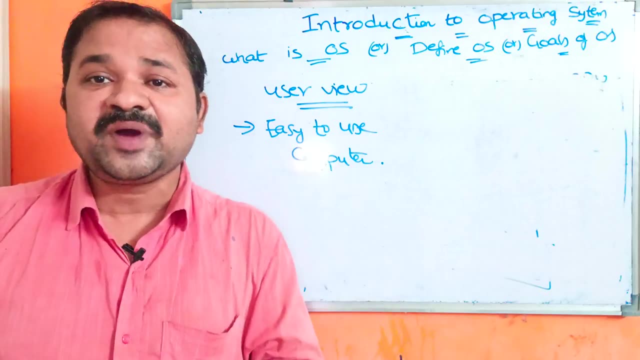 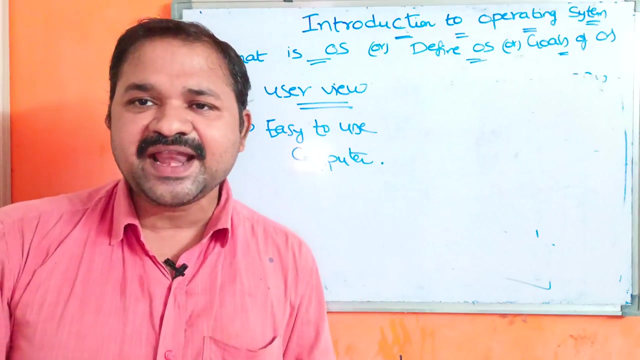 it is the responsibility of the operating system to transfer that program from hard disk to main memory. so if we have given some print out print out, then it is the duty of the operating system to allocate the printer. so if you want to do some scanning then it is the responsibility of the scanner operating system to allocate scanner to 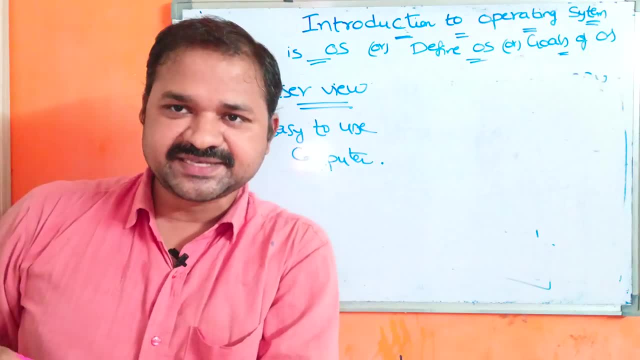 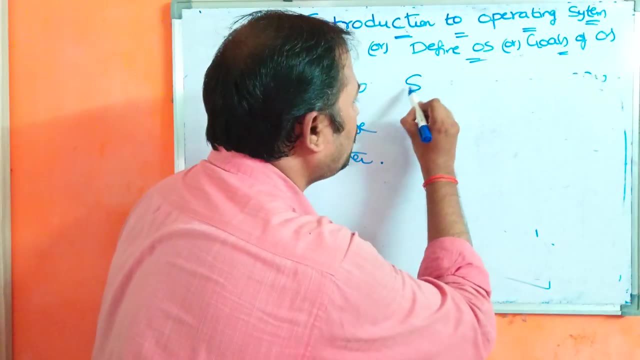 our file. so everything will be taken care by the operating system. only so we can use the computer very, very easily with the help of the operating system. now let us see what is operating system from system point of view. from system point of view, what is an operating system?